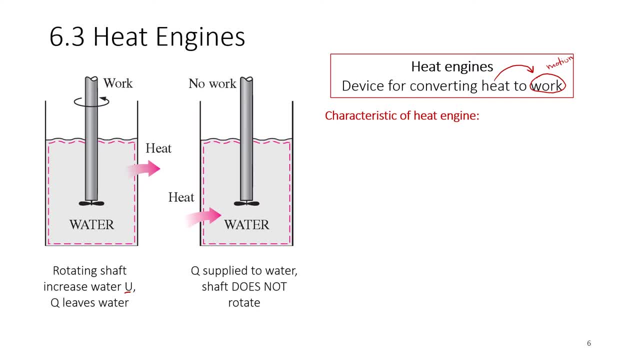 And the heat will leave the water. So if you rotate this shaft, the energy of the water will increase. Energy in what form? Of course we're talking about internal energy. Okay, it will increase. And then if the let's say this is not an insulated system, 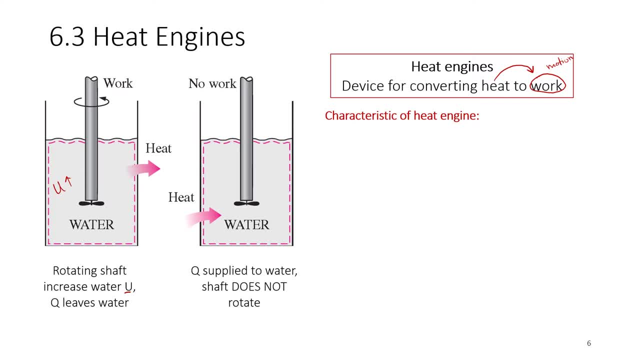 the increase will cause an increase in temperature And therefore heat will be transferred out to the surrounding. This is a natural process. It follows the first law, It follows second law. But what if you want to do the opposite? So you heat up the water? 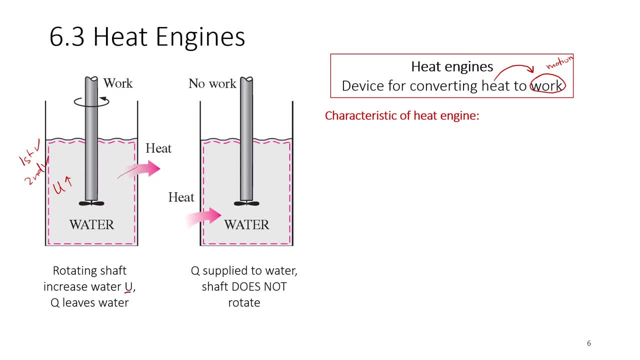 And then suddenly, magically, the shaft will turn. No, that's not going to happen, Right? So we need the device like heat engine in order for this to happen. So characteristics of heat engine: They receive heat from a high temperature source. 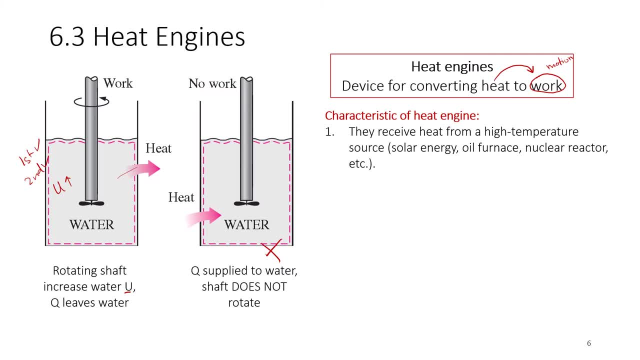 Okay, high temperature source can be solar energy, can be oil furnace, can be nuclear reactor And, like I said, the previous topic- it can be the sun. Okay, anything at all that can be considered as a thermal reservoir, So it will receive heat from that. 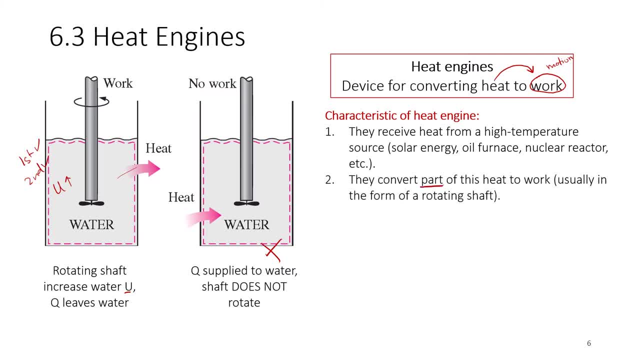 And it will convert part of this heat to work, And normally when you talk about work, it's usually in the form of rotating shaft. Okay, it converts part of this heat. Yeah, that's the key word here: Part of it, not all of it. 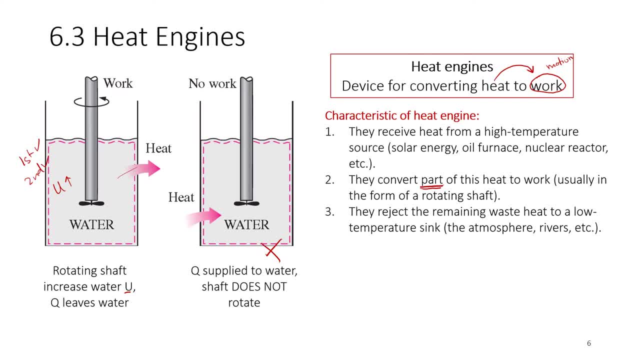 And then what happens to the rest of the Heat? They reject the remaining waste heat to a low temperature sink. Okay, so part of it becomes work. There's a remaining heat we call waste. Waste means something you cannot use anymore. 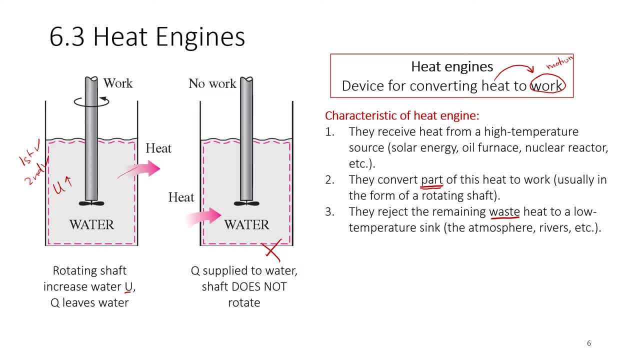 Rejected to the low temperature reservoir or the sink. And finally, most important part, they operate on a cycle, So it's not a one-off process. It has to operate on a cycle for you to get continuous supply of work. Okay, so these are the characteristics of a heat engine. 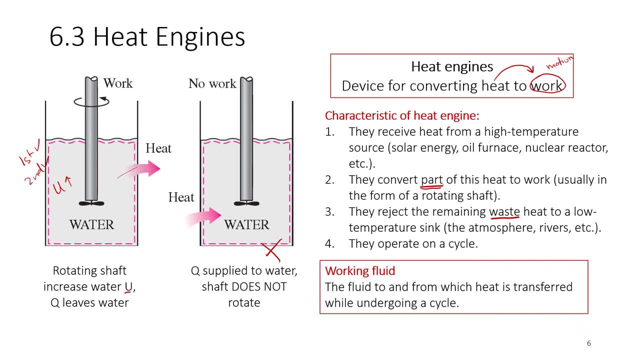 And in order for this to happen- for it to operate on a cycle- there has to be a working fluid. What is a working fluid? A working fluid is the fluid to and from which heat is transferred while undergoing a cycle. So there's a cycle. 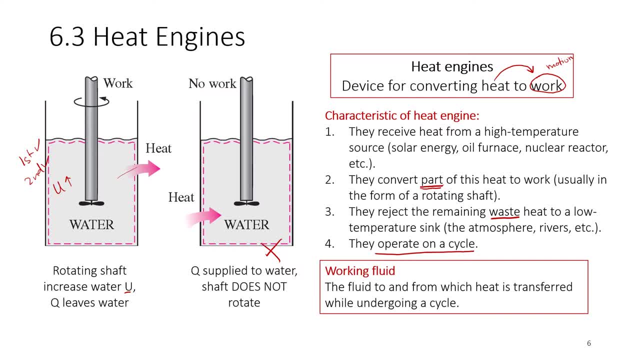 Just think about a system like your aircon system or your car. Okay, so all the devices are working. You can't just have one device. You need to have all the devices In aircon, for example, you need compressor, You need the. what do you call this? 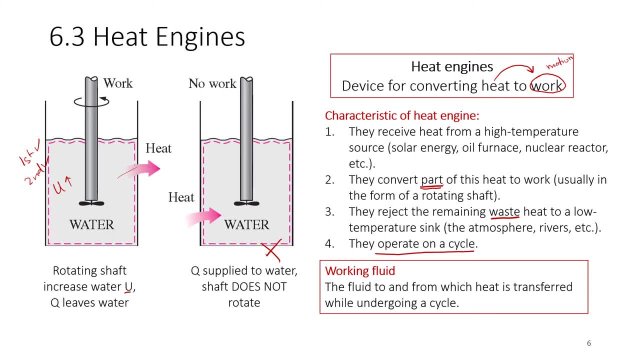 The pump. Okay, so how are these devices connected? So the working fluid is what connects them. Okay, so you will see in specific system what kind of working fluid are we referring to. Right, so that's the introduction to heat engine. 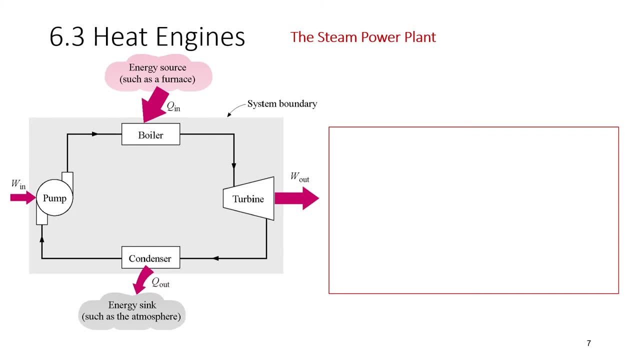 Okay, so what you are seeing now here, the diagram on the left- is a schematic diagram of the steam power plant. Okay, we're going to go to the diagram one by one, But let's look at the definition first. Steam power plant is an external combustion engine. 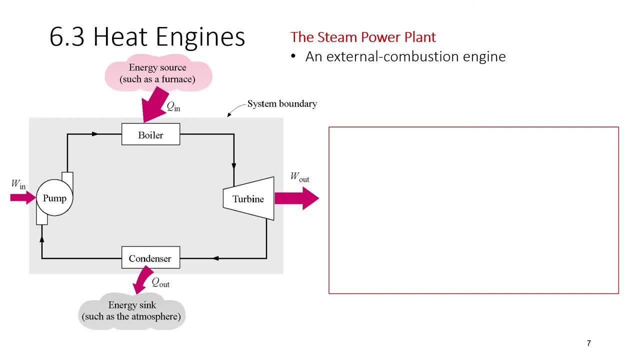 What is external combustion engine? It means that the combustion is happening outside the cycle. Okay, combustion takes place outside the engine. Thermal energy release during this process is transferred to the steam as heat. Okay, so when you look at this diagram, the combustion is happening in the furnace. 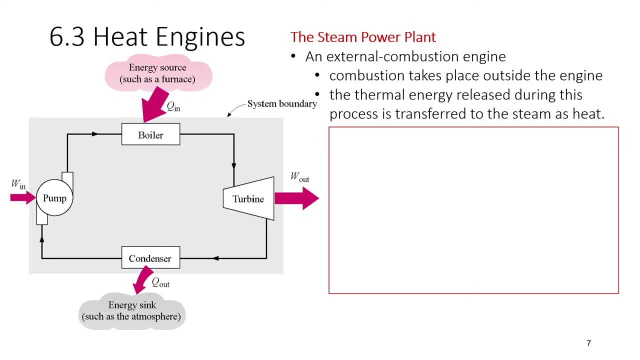 Okay, so the furnace is the source energy source, the reservoir And the sink is the energy source and the sink is maybe just the atmosphere. so let's look at the entire system. so the plant is the whole thing, you see, heat engine, it is the whole thing, it's not just one device. 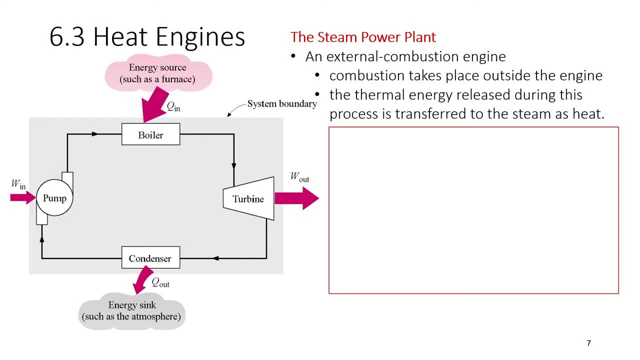 okay, it's made up of different devices, okay. so what happens at each stage? let's see okay. first, you um ignite the furnace, so the furnace is on, it supplies heat, cue in, it supplies heat to the device called the boiler. so what happens in a boiler is: this is a steam power plant. therefore. 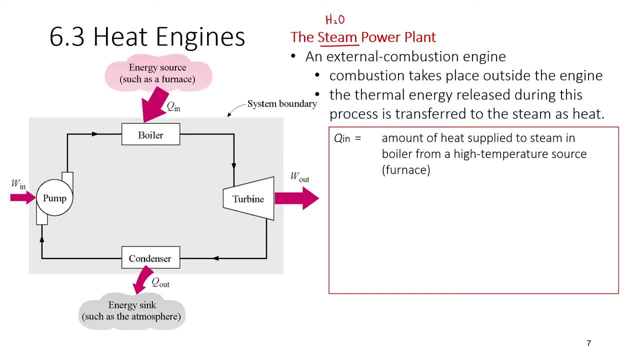 the working fluid is water. what happens when you boil water? it turns into steam, obviously, okay. so at this process, amount of heat supplied to the, to the steam in boiler from a high temperature source, that is cue in. okay. so now you have nicely converted this water to steam, so it follows this path. look at the arrow. 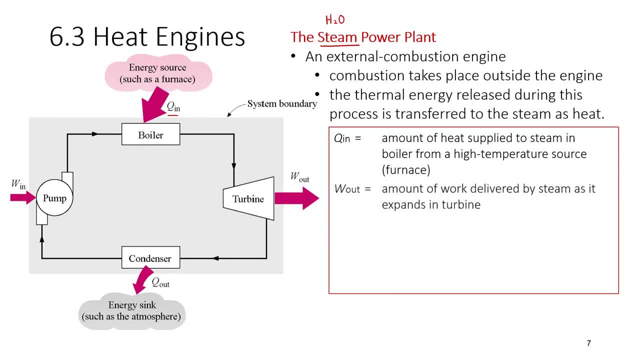 yeah, it goes into the turbine. what happens in the turbine? a steam has very high energy. what it does is it will rotate the blades in the turbine. okay, it will rotate the blades in the turbine and produce work output. how the blades in the turbine are connected to a shaft, so here there will be a shaft coming out of the turbine. 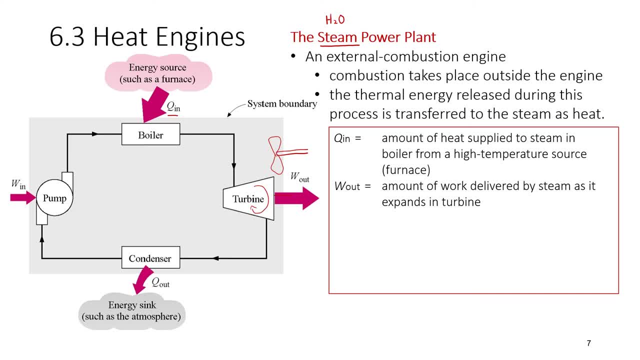 normally connected to generator. but we don't touch that point, we just want to produce the work output. So a shaft, rotating shaft, considered work output. Okay, so work out is the amount of work delivered by the steam as it expands in the turbine. Okay, as it rotates the turbine blades. 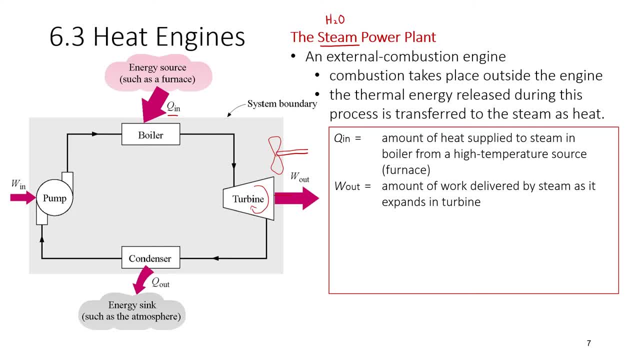 So what happens to the steam next? It exits the turbine, obviously with different properties. now It has spent all its energy here. You've learned this in Chapter 5.. It's turbine and compressor, remember. So turbine is opposite of compressor. 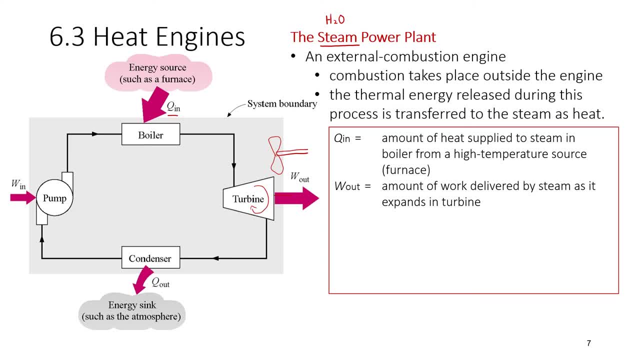 So the pressure will be different, the temperature will be different as it comes out. So it comes out, it has to enter the device called condenser. So condenser- how to remember what it does? It condenses. Condenses means 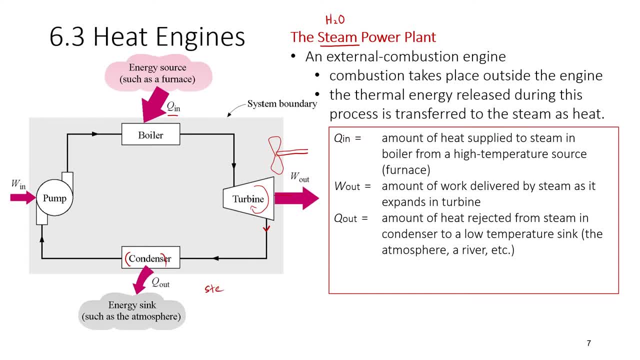 It condenses: turning from steam to liquid. condensation or vapor turning into liquid. How to turn vapor into liquid? You cool it down. How to cool it down? Reject heat, remove the heat. Okay, how to remove heat? Put it in contact with something that is colder. 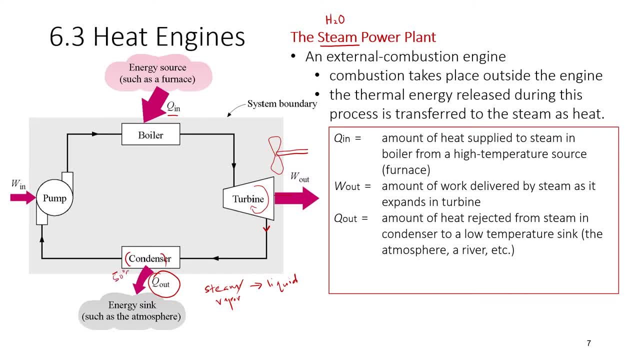 Let's say this is 50 degrees, this is 30 degrees. automatically heat will be transferred. Okay, so your steam coming out from the turbine will be condensed. So Q out refers to the amount of heat rejected from steam in the condenser to a low temperature sink. 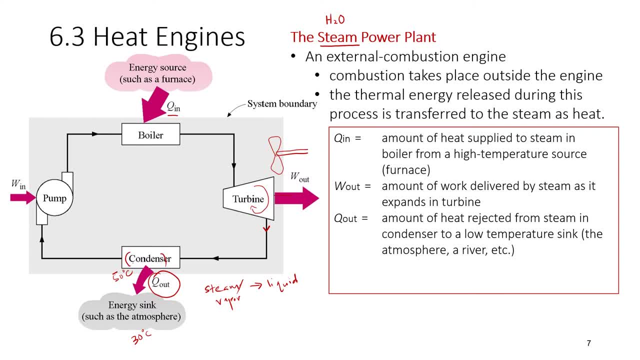 That sink can be anything: Atmosphere or a river, etc. So it doesn't matter. That is not for us now to understand this theory. It doesn't matter, Okay. so after the condenser, the liquid. now, okay, the liquid water has to go to the pump. 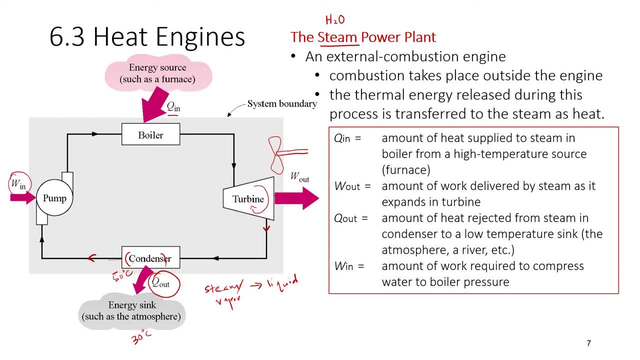 Because there is some work in that needs to be supplied. Amount of work requires two conditions: Compressed water to the boiler pressure. So the water that comes out from the condenser has low pressure. In order for it to complete the process and repeat the cycle, it has to match the pressure here. 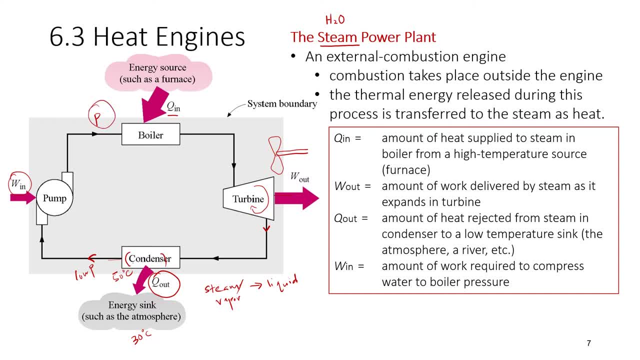 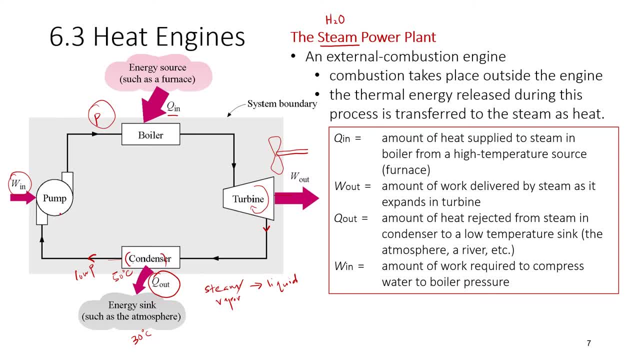 The pump will increase the pressure and then you can send the water back to the boiler and the process continues. Okay, An important equation. I hope you write this down as you watch all these videos. The net work output produced is equal to, of course, work out minus work in. 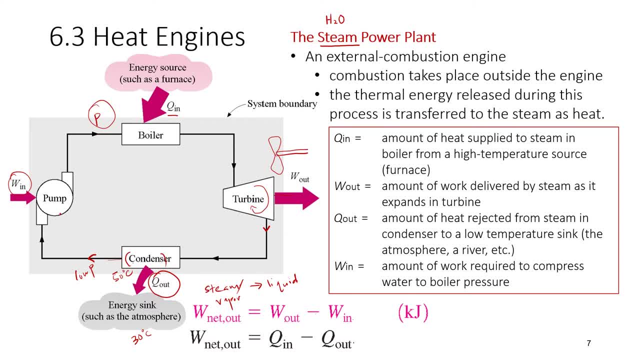 This is energy balance. Okay, the net work: work out minus work in, or? this is also very important. Write this down. In the case of this heat engine, you can write it as Q in minus, Q out, Okay, Okay. 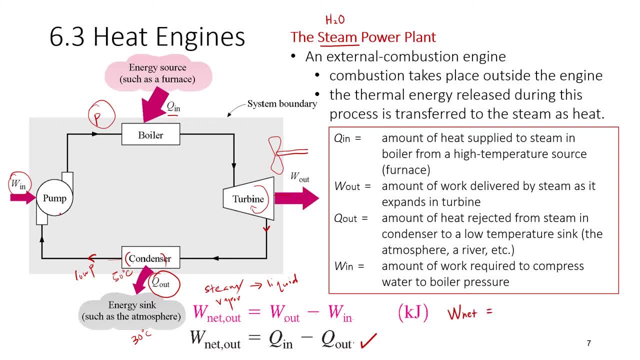 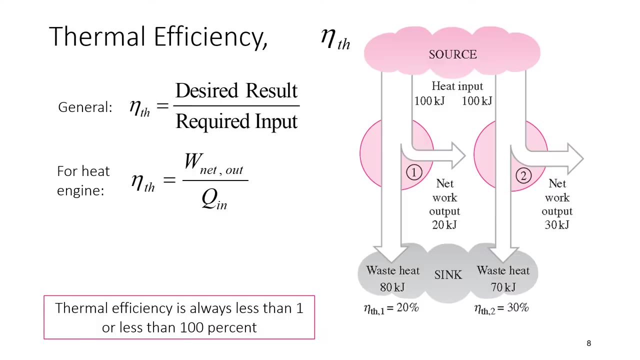 Okay, Okay. So net work equals to: you can write it like this: So write this equation first under heat engine. This is how we can calculate how much work is being produced by the entire system. Okay, Next we come to the thermal efficiency. 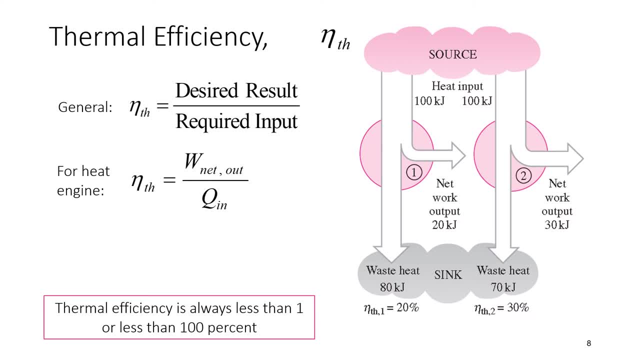 Okay, Any device has an efficiency. Okay, And the efficiency, the general equation, you see this: and Th means thermal efficiency. The symbol nu means efficiency, Th means thermal. Okay, So when you talk about heat engine, you're talking about the thermal efficiency. 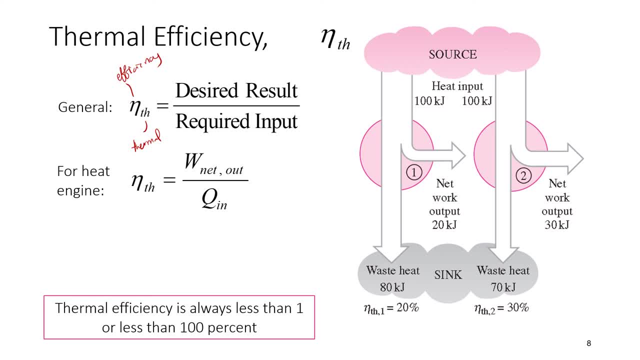 Okay, Okay, So this is thermal efficiency, Right. so generally, efficiency is desired result, or in other words, what you want over required input. okay, required input is what you pay. all right, that's a general equation for efficiency: what you want from the system, or what you're getting from the system, divided by what you have to pay to get it. 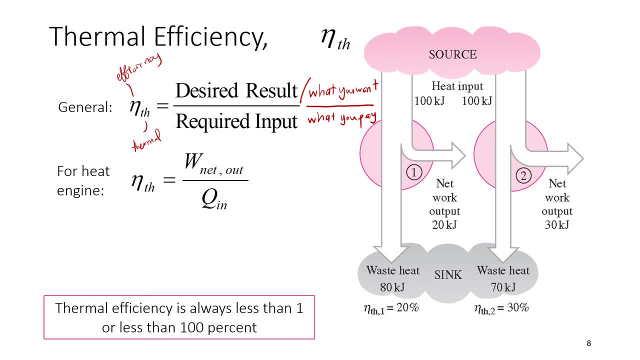 so, for heat engine, what do we want? of course you want work output, okay, so we put that at the top: work output. that's the whole thing point of having a heat engine. what do you have to pay? you have to supply the heat source, so divided by what you pay is the Q-in. so this is the equation for heat engine's. 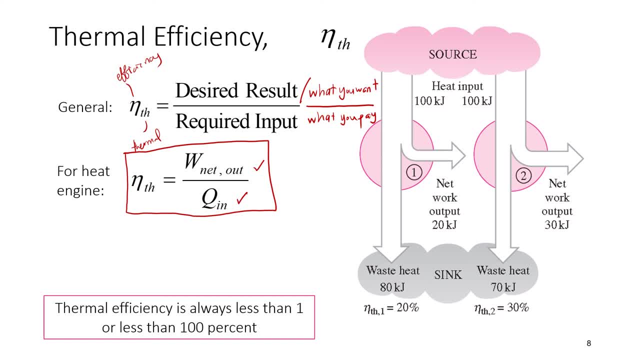 thermal efficiency. write this down as well. okay, and it says here that thermal efficiency is always less than one. or look, if you use percentage, always less than 100 percent, always. why? why is it not 100 percent efficient? because we have to reject heat. there's still some waste, so the waste is causing the 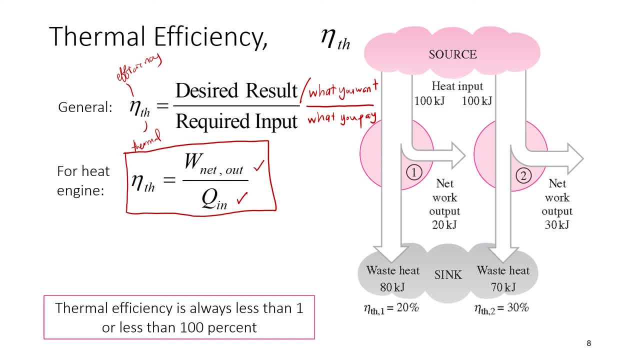 efficiency to be less than perfect. okay, so if you look at this diagram, we have the same source- source means heat source. we have the same sink that will absorb the waste heat, and then we have two different heat engines, one and two. so the source supply, the same amount of heat: 100 kilojoule. 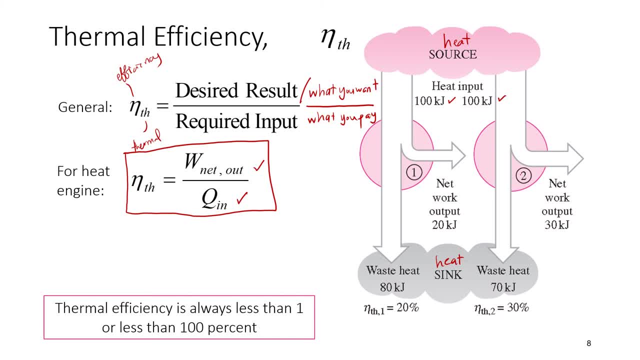 heat engines, one and two, because they are different. they produce a different work output. this one produced 20 kilojoule only. this one produced 20 kilojoule, only produce 30 kilojoule. so what about the waste? the waste is as simple as the waste. heat is 80. 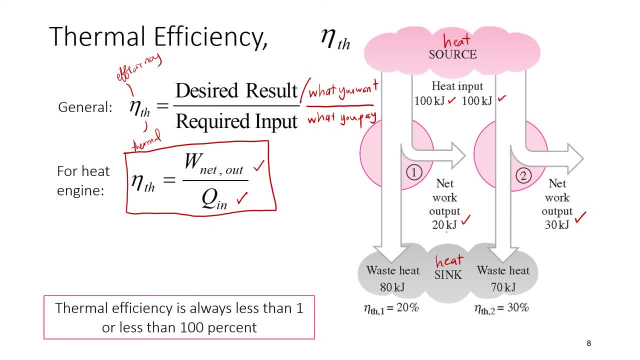 because 100 minus 20, you get 80, and for the other one, 100 minus 30, 70. so which one is better? the one that produces more work and it shows in the thermal efficiency. this is the thermal efficiency. 30 percent efficient. this is 20 percent efficient. okay, very simple. so this is calculated thermal. 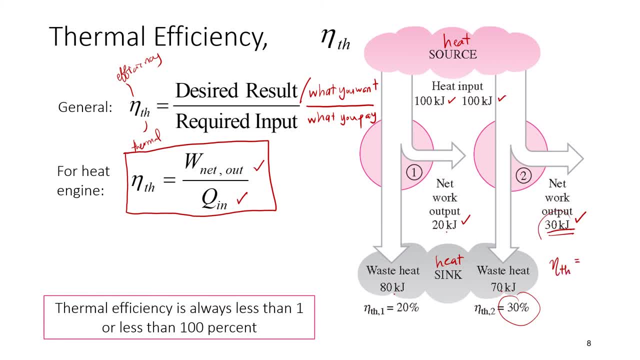 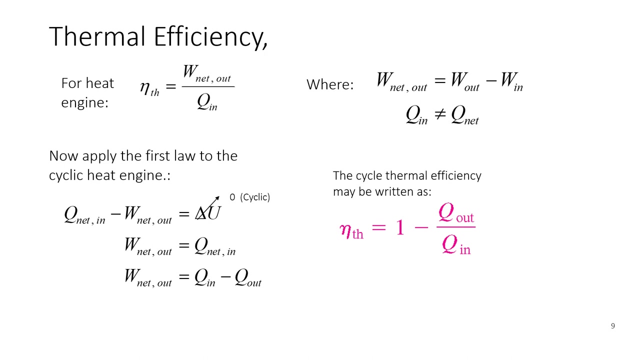 efficiency. what you want here is the work output, 30 kilojoule. what you pay is 100 kilojoule. the Q in, therefore, this is 30 percent. very, very straightforward calculation. okay, this is an quite an important slide. so what can we do with the equation? so for heat engine: 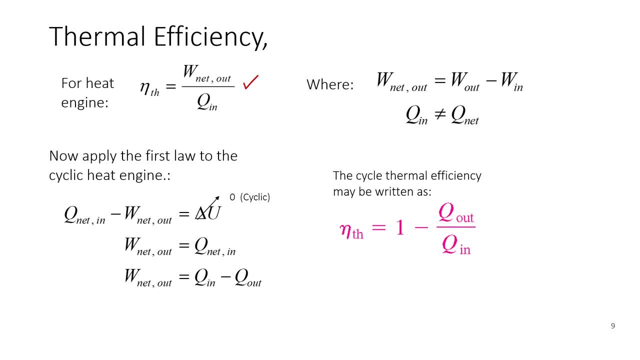 you've seen this. what you want work output, what you pay is a heat supply. okay, to keep. to make it simple, I'm going to lead you to this pink equation. so what happens here is we replace this part, this portion, with Q in minus Q out. you saw, in the previous slide I asked you to write down Q in. 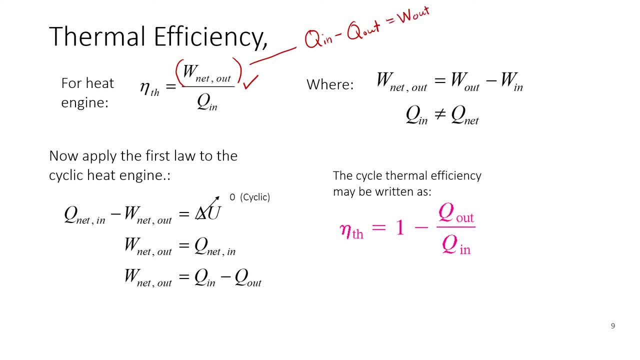 minus Q out equals to work output. so we can replace this. so what happens when replace it? thermal efficiency becomes Q in minus Q out over Q in. becomes Q in minus Q out over Q in. This equation becomes this: Q in minus Q out over Q in. 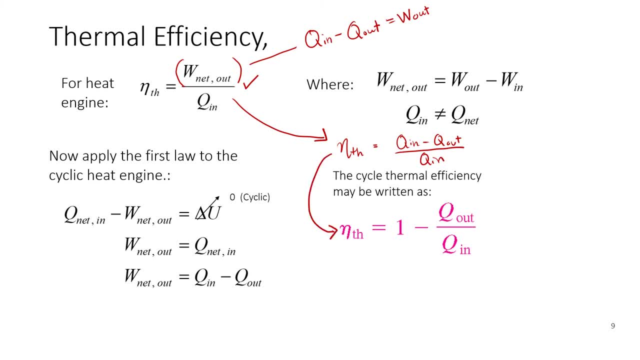 And this can be written as 1 minus Q out over Q in: Okay. so same equation, One version. you can use it this way. you can use it this way, Okay. so in some cases, let's say, you have to calculate, you don't have the work output. 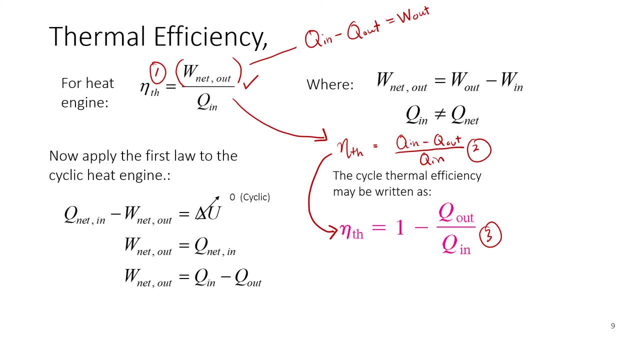 You have Q in and Q out, so you can use this version. What's most important, I suggest that you understand what it means. The efficiency is what you want In a heat engine. what you want is the work output. What you pay is the heat source. 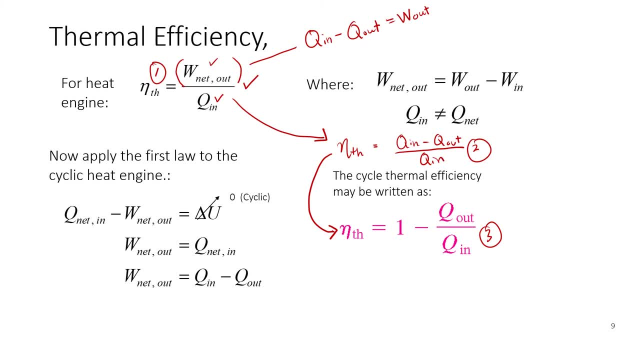 So from that understanding, you can easily figure out how the equation should be. And, of course, you have to also understand this, The same thing that we have here. This is how we get it from the energy balance equation. Okay, remember this. 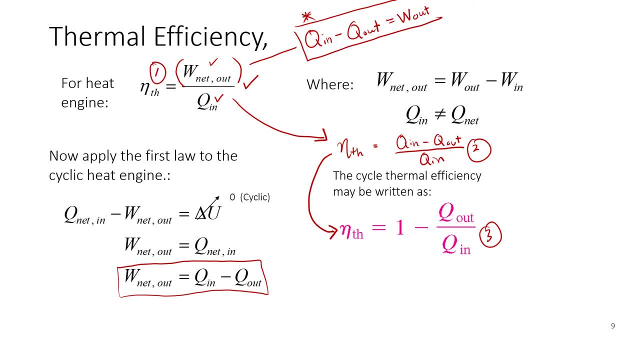 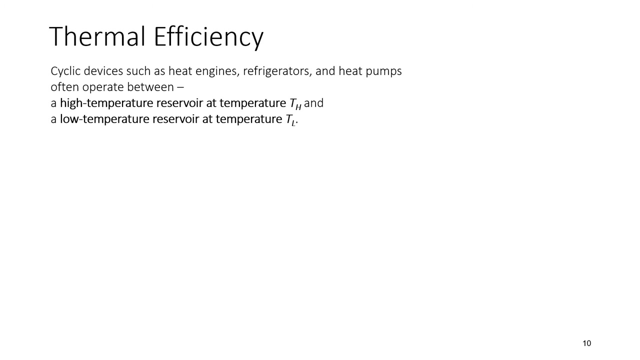 Understand what is efficiency and you can work out these equations. Okay, as this is a recorded lecture, you can pause anytime you want to write things down or whatever, So I'm just going to proceed. This slide will show you cyclic devices such as heat engine, refrigerator and heat pumps. 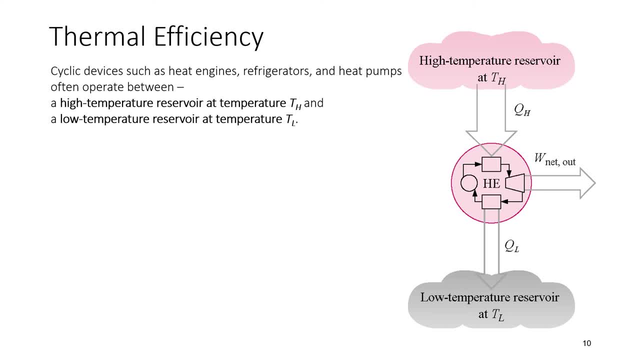 often operate between high temperature reservoir Label as TH for temperature high, and a low temperature reservoir. at temperature TL stands for low temperature. Okay, so what does that mean? This is your heat engine, We have the boiler, we have the turbine, condenser and pump operating in a cycle. 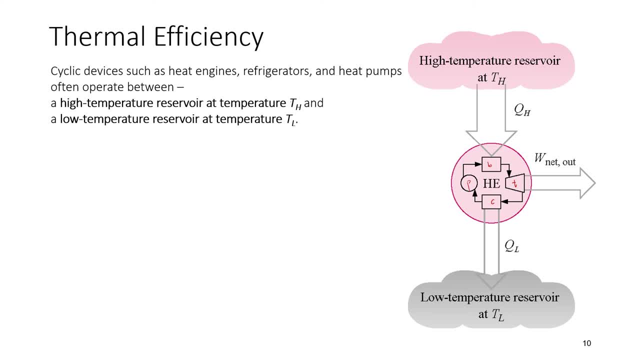 As I said just now, this whole thing is considered one device. It's a cycle. As I said just now, this whole thing is considered one device, It's a cycle. As I said just now, this whole thing is considered one device. 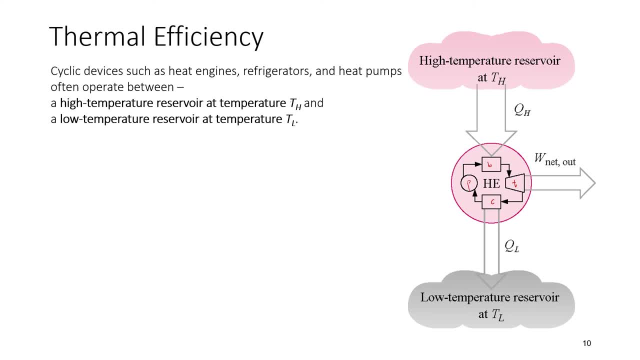 It's a system, So we have our source, heat source. It has to be at high temperature. That's why TH. This is not heat, this is high, high temperature, And then it produces work fine, And then it rejects the heat at low temperature TL. 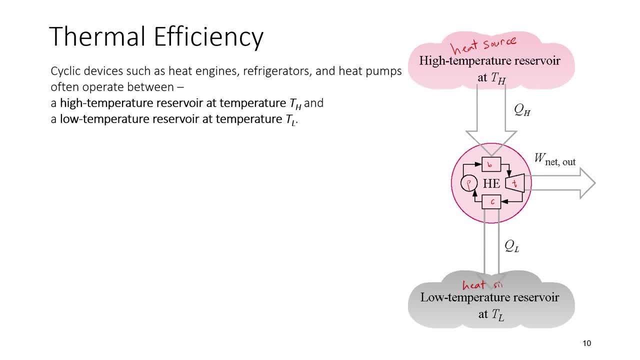 So this is your heat sink, Okay, so instead of calling it Q-in and Q-out just now- we said this is Q-in, this is Q-out- We are going to call it Q-H and Q-L. Okay, Q-H does not mean high Q. 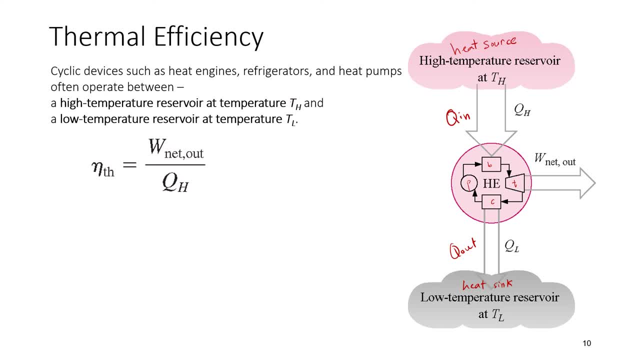 And this is low Q. no, Q-H is the Q-L, Q-H is the Q-L, Q-L is the Q from the high temperature source. Q-L is the heat that is transferred to the low temperature reservoir. So the letter L and H refers to the temperature of the reservoir. 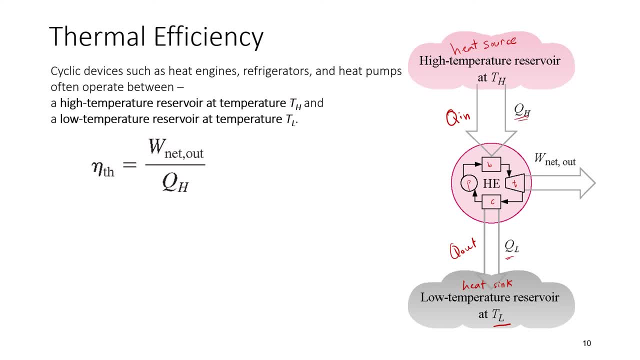 Not exactly the amount of the Q. Okay, don't get mistaken about that. So, based on this diagram, efficiency- what you want is this part, So we write it at the top. What you pay here, what do you have to pay, is Q-H. 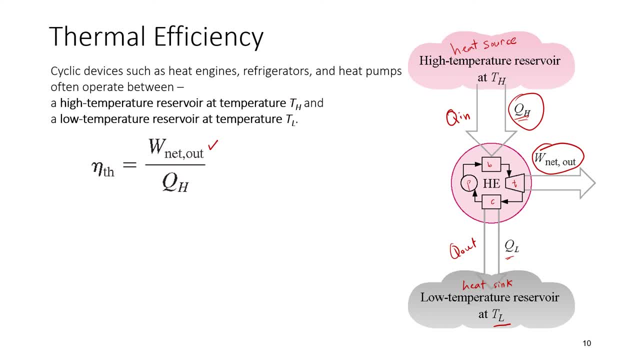 So that's your equation. So you see, if you understand, you can get different versions of it. So the net work output is: instead of Q-in minus Q-out, we write it as Q-H, Q-H minus Q-L. Okay, Q-H minus Q-L. 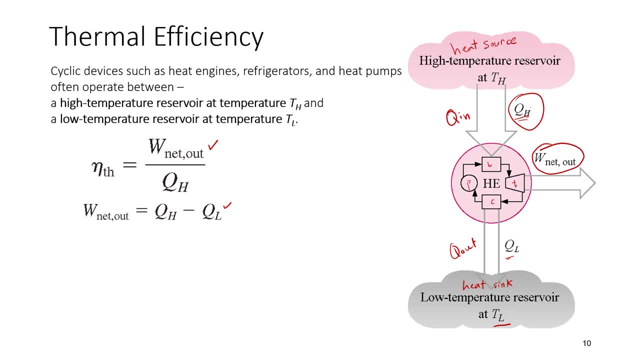 We're just replacing in and out with H and L. Okay, so the equation for the thermal efficiency. you can write it as 1 minus Q-L over Q-H. How do we get this From this equation? we get this version. 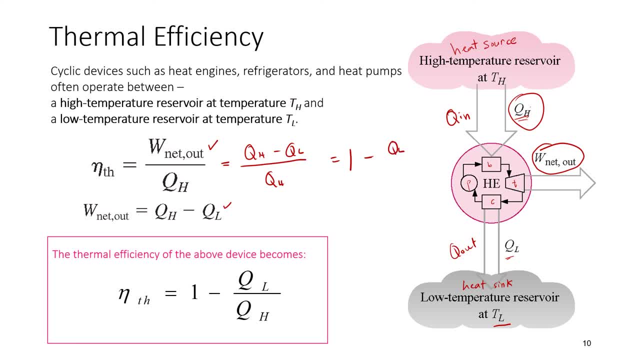 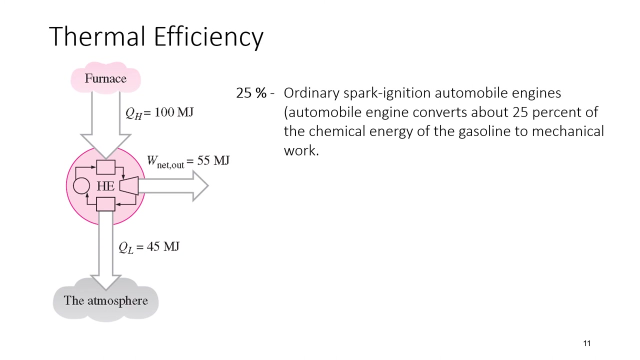 Q-H over, Q-H becomes 1.. Okay, so we get this one. You can use whichever version according to the suitability of the question later on. Okay, Okay, Let's look at some examples of what kind of values of efficiency do we get from devices around us? 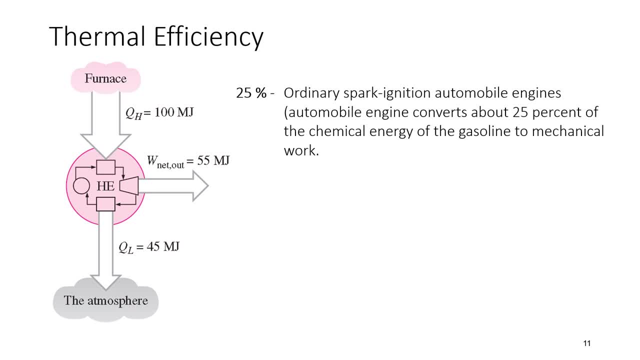 Okay, Ordinary spark ignition automobile engine: your normal car engine is 25% efficient. Okay, not as high as you imagine, right? If it's a diesel engine, 40%. Large gas turbine plants also 40%, Okay, Okay. 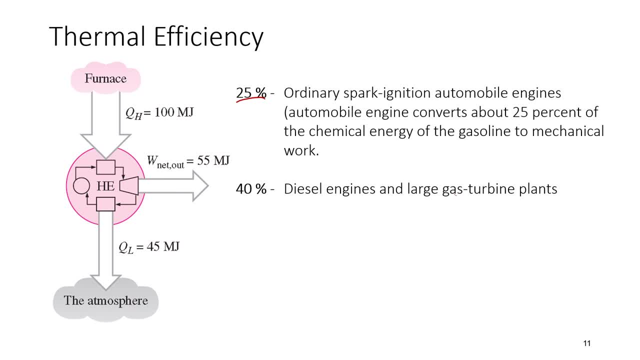 Okay, Okay, Okay, Okay. What is a gas turbine plant? Okay, means the plant operates with gas as a working fluid. Just now we saw steam was a working fluid. Okay, 60% efficiency if it's a large combined gas and steam power plant. 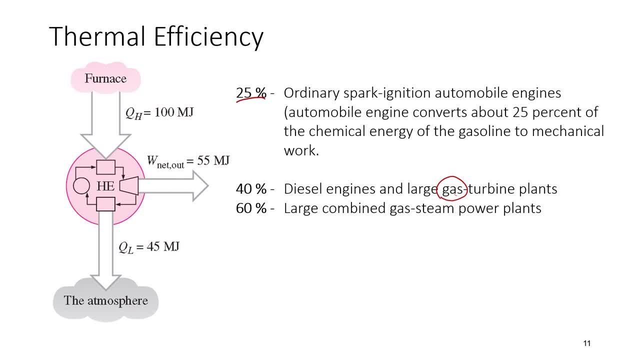 Okay, the power plant is in a large scale and it combines gas and steam as the working fluid. This has a high efficiency. So what does that mean? These are not very good numbers. Almost one half of the energy supply ends up in the rivers, lakes or atmospheres as waste. 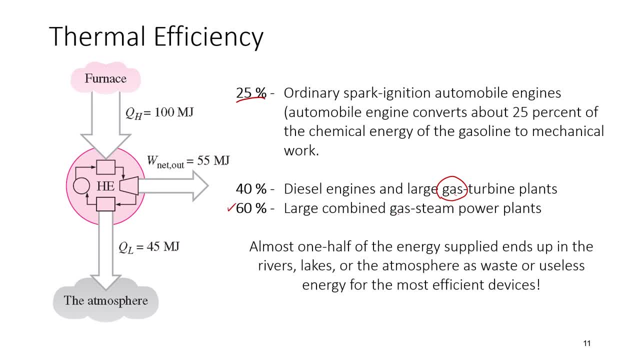 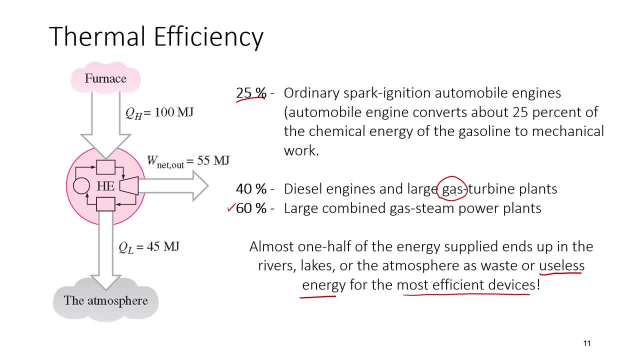 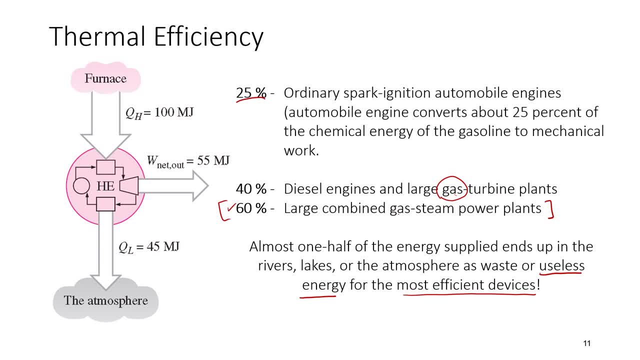 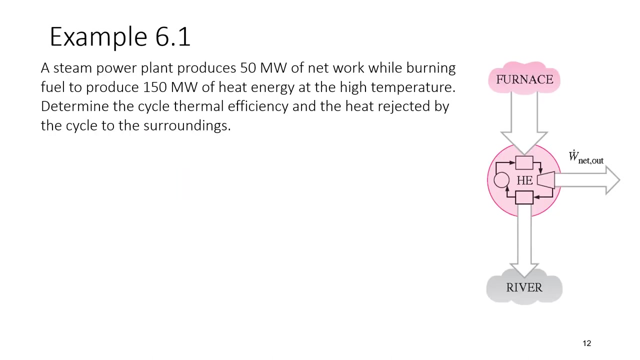 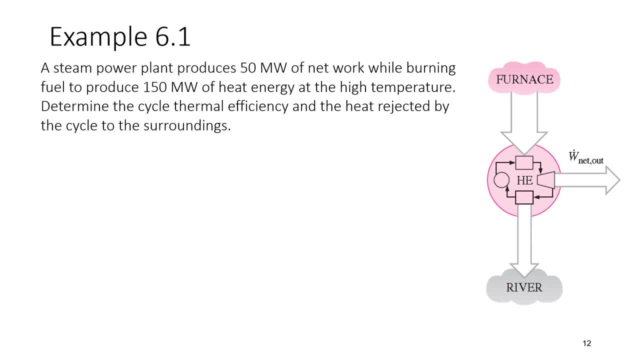 a steam power plant produces 50 megawatt of net work. get used to writing it down: megawatt, okay, network. so even though it's called work, the unit is what. so it has a dot. this is the work output while burning fuel to produce 150 megawatt of heat energy at the high temperature. 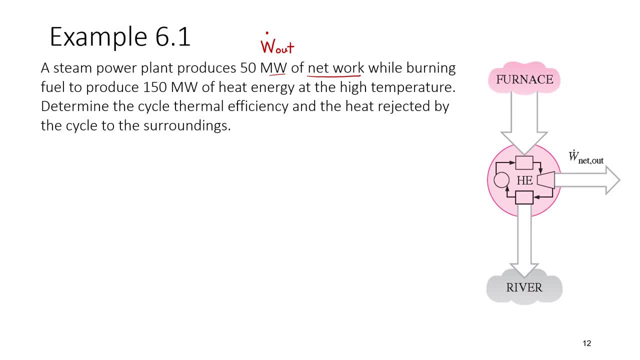 so you need to produce 150 megawatt of heat energy in order to produce this work output. So 150 is the Q H here. 150 megawatt coming from the furnace Determine the cycle, thermal efficiency and the heat rejected by the. 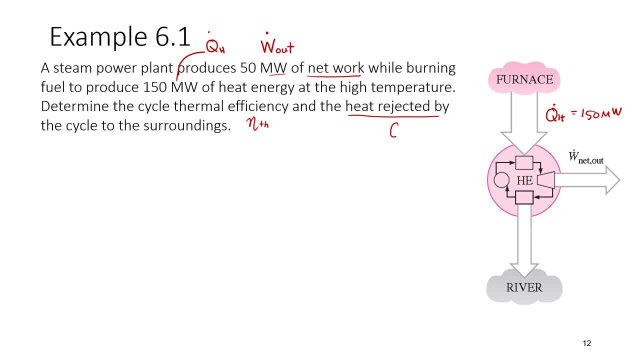 cycle to the surroundings Heat. rejected Q L here. Very simple question: Thermal efficiency. we have this equation. What you want in the heat engine again is the work output. I should put a dot there. What you have to pay is the heat. 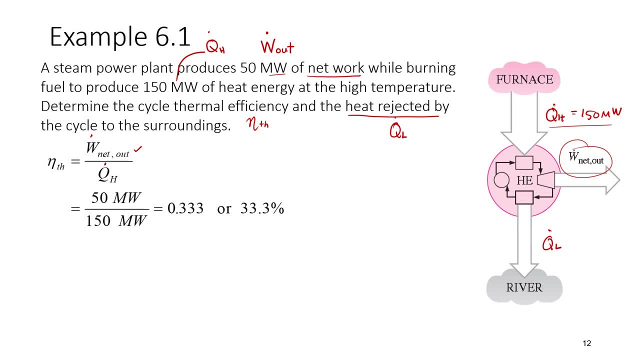 source heat supply In 33% or 33.3%. This is the efficiency. Okay, the next part is heat rejected Q L. So what equation do we have? Work output is equal to Q H minus Q L. Very simple: You can add a dot here to show that you're talking about rate. 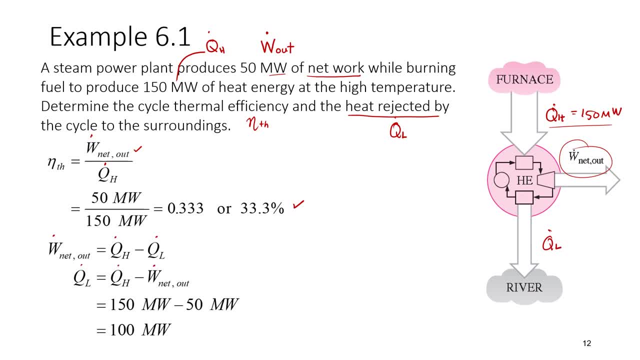 Okay, so Q L is just 150 minus 50, 100 megawatt. So 100 megawatt is being rejected. Okay, very straightforward application of the equations. Okay, another one. Here we have the heat output. Here we have the heat input. 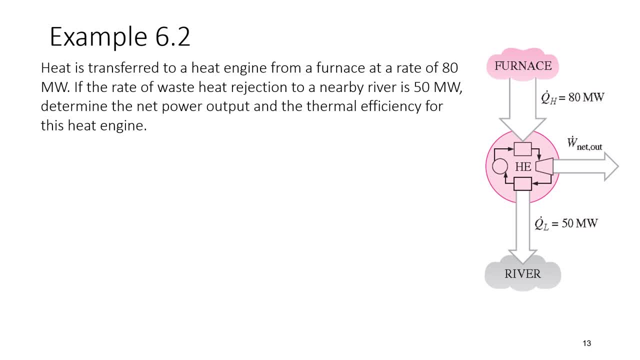 heat is transferred to a heat engine from a furnace at a rate of 80 MW From furnace. so that means this is the source, Not always that you have a diagram like this. so you have to know how to place all these values If the rate 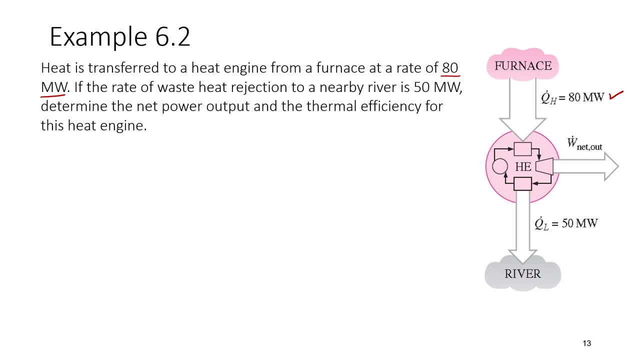 of waste heat rejection to a nearby river is 50. obviously this is QL. Determine the net power output, work output and the thermal efficiency. You have QH and QL. you can obtain work output very easily. Just use this equation: Work output QH minus QL. 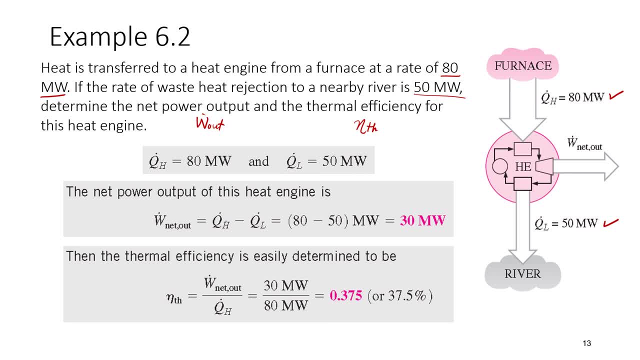 Once you have the work, you can calculate efficiency using this equation: Get 37.5..